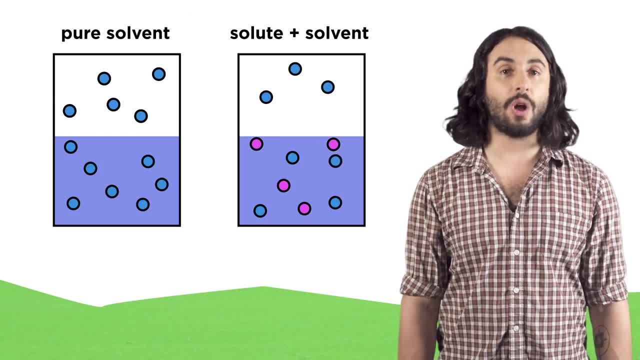 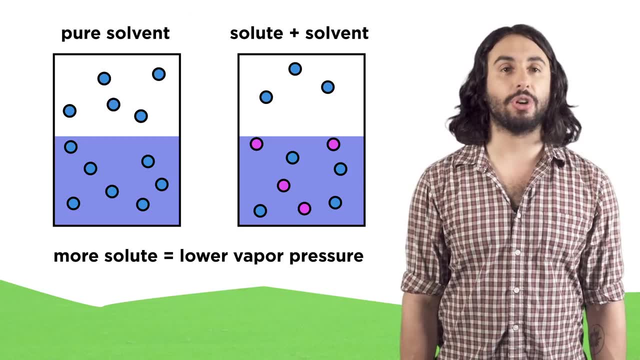 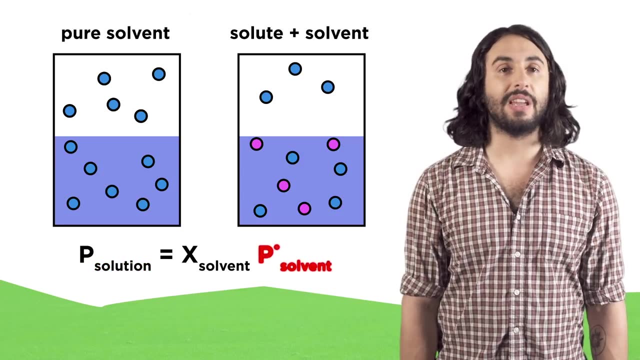 which hinders some solvent molecules from evaporating. therefore, the presence of the solute causes the vapor pressure of the liquid to decrease. the new vapor pressure is equal to the vapor pressure of the pure solvent times the mole fraction of the solvent which refers to the 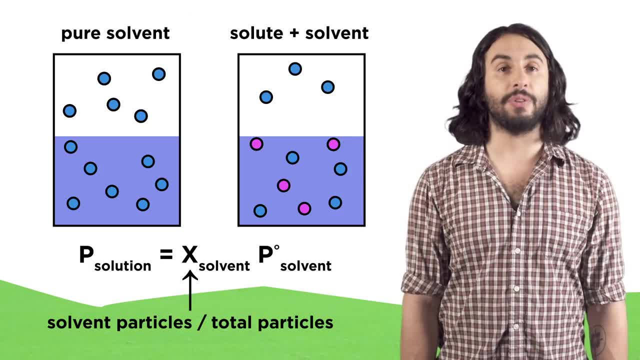 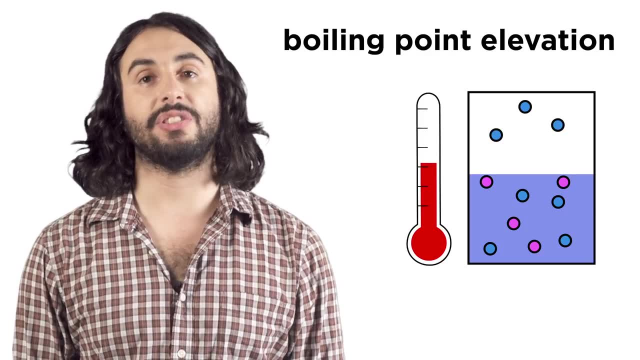 percentage of particles in a solution that are solvent molecules. a similar phenomenon is that of boiling point elevation. when we look at a solute, we can see that the vapor is constantly changing when a solution is raised to the temperature at which the solvent 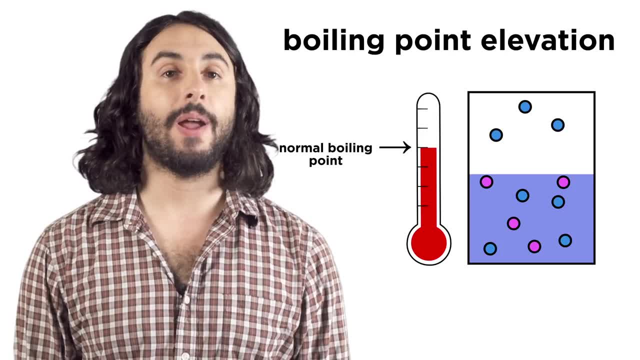 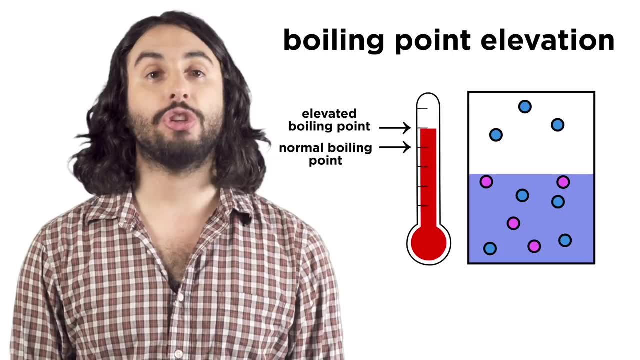 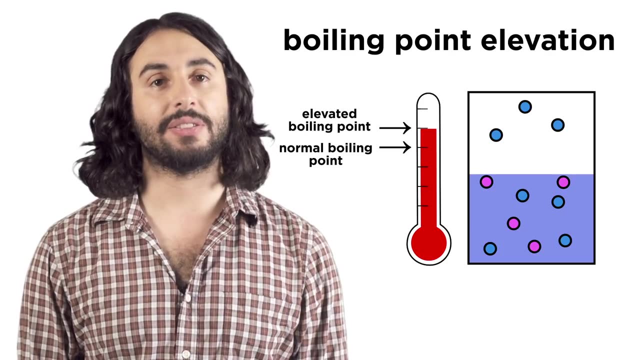 should boil again. there are solute particles blocking the solvent molecules from going into the gas phase. this means more heat energy will be needed to compensate for this activity, which results in an elevated boiling point. the more solute there is, the more dramatic. 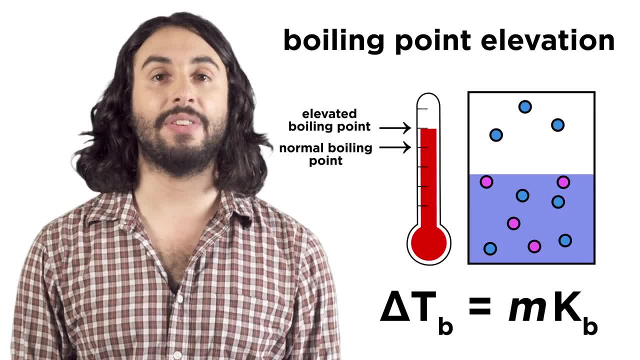 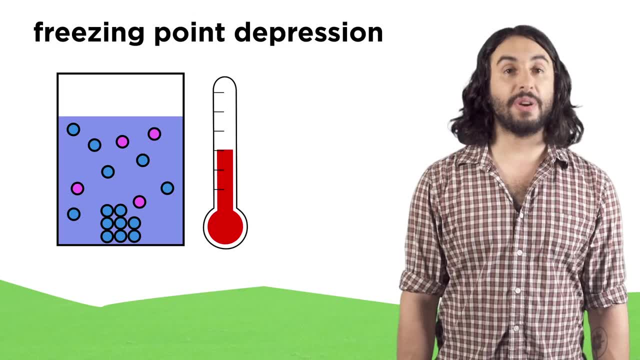 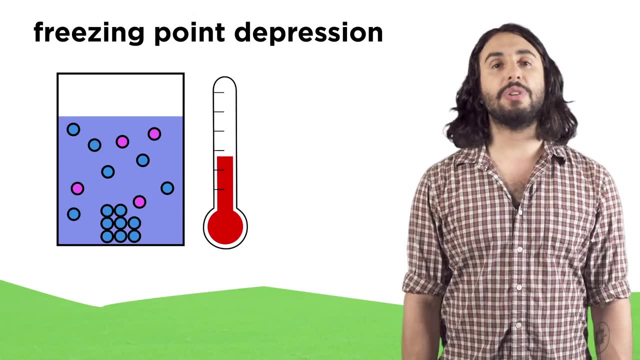 the effect. so the change in boiling point is given by the molality of the solution times, a constant that is specific to the solvent freezing point. depression is similar but deals with the interface between the liquid and solid phases for a liquid to freeze 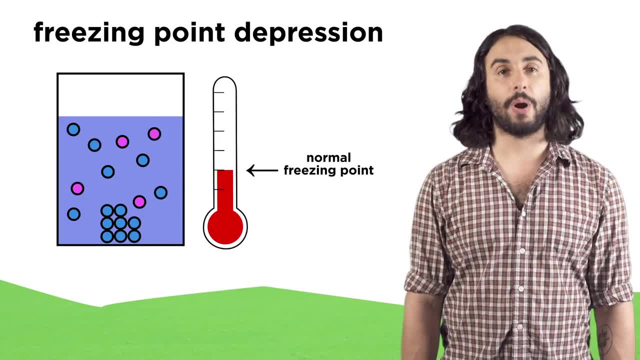 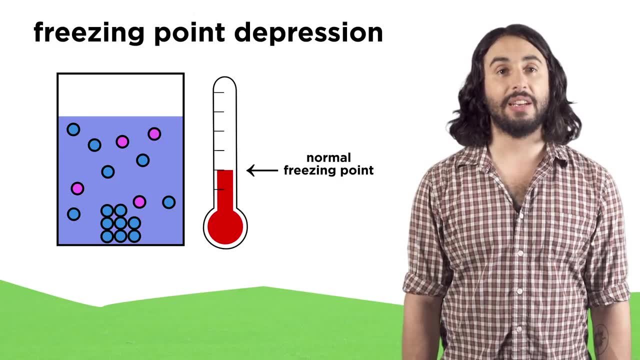 it has to form a lattice. the presence of solute particles interferes with the ability of the solvent particles to efficiently form the lattice, so to compensate, the system will have to reach an even lower temperature to freeze. the equation here is similar: the change in freezing point is the activation of a liquid into a solid. we speak of an air, but we will now explain a solute. in a solute, the presence of a solute has to be greater. solute has to be greater than the air temperature. only in a solute the temperature of the liquid 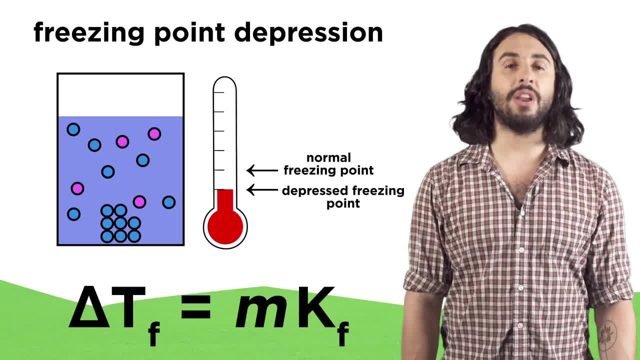 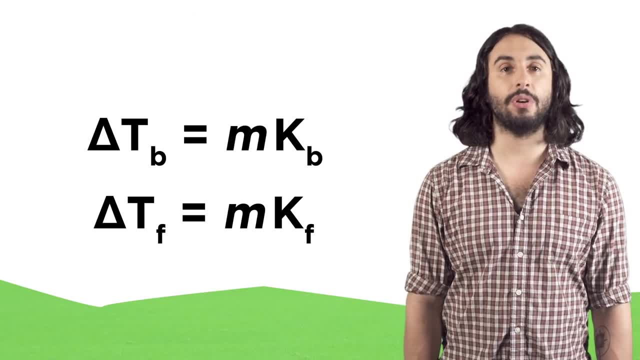 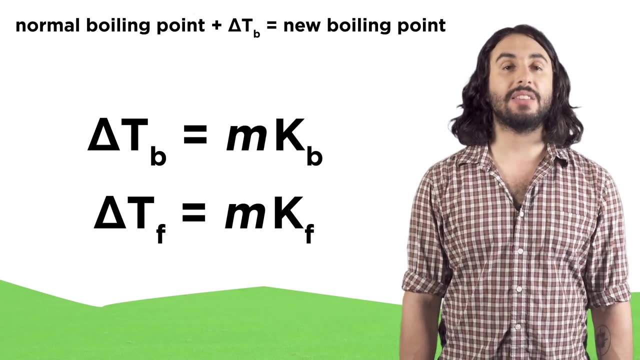 is given by the molality of the solution times another constant. these KB and KF constants can be found in tables in your textbook or online. remember to always add the change in boiling point to the original boiling point, since solute always raises the boiling point and change in freezing point will always be. 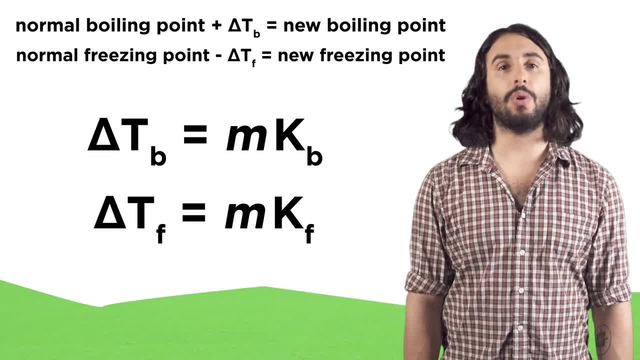 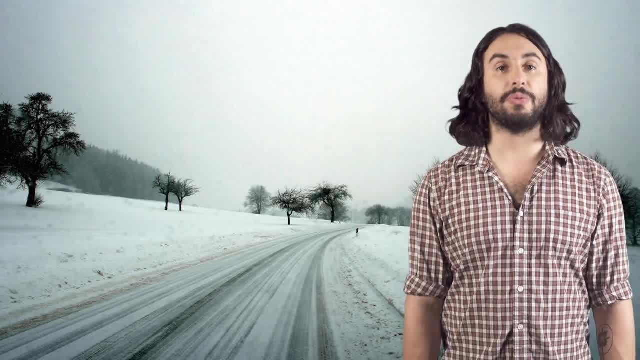 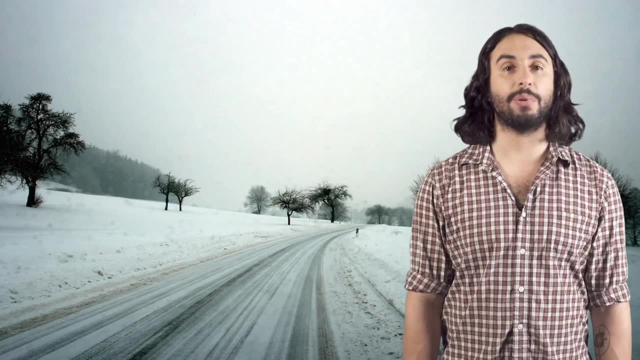 subtracted from the original freezing point, because solute always lowers the freezing point. this is why we add salt to icy streets, because it causes the water to freeze at a lower temperature, so water will remain liquid instead of turning to ice, until lower temperatures are reached, thus reducing the quantity.